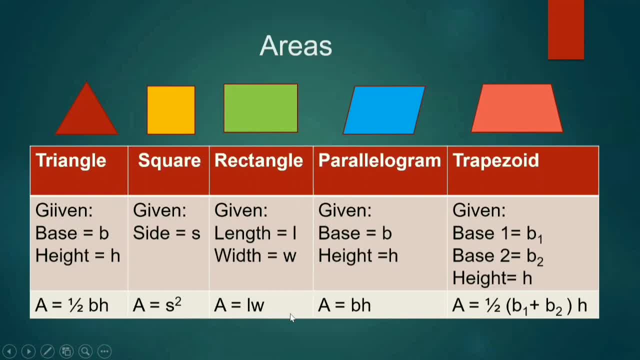 Rectangle Area is equal to length times width, Parallelogram Area is equal to base times height And trapezoid Area is equal to one half of base 1 plus base 2 times the height For the volumes we have. the volume of a cube is equal to: 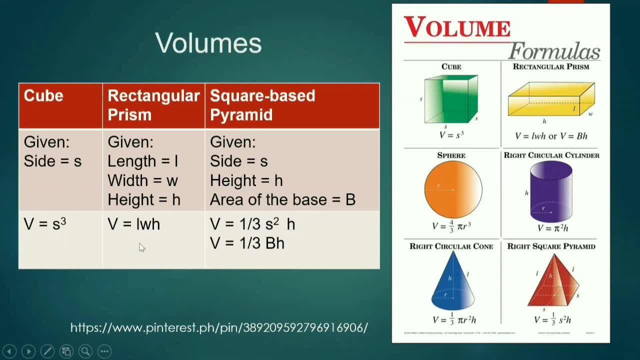 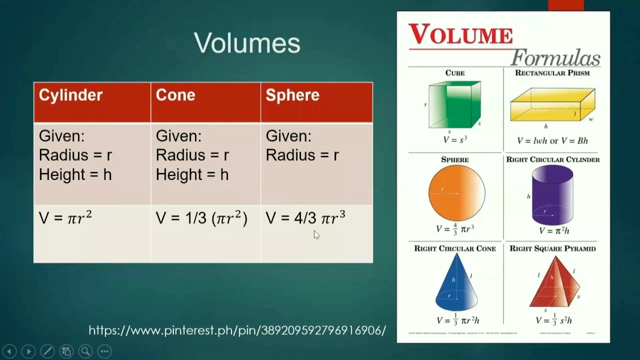 S cube, The volume of a rectangular prism is equal to length times width times height, And the volume of a square base pyramid is equal to one third of the area of the base times height, or one third of S squared times height For the cylinders. 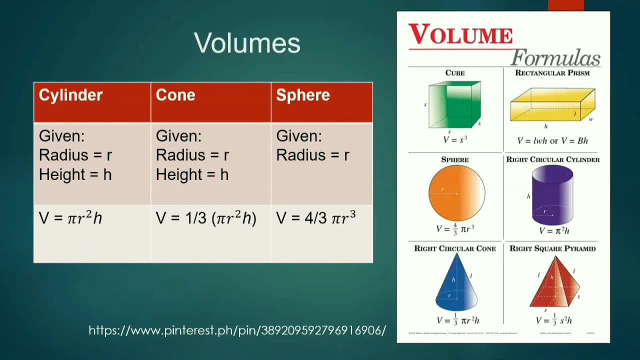 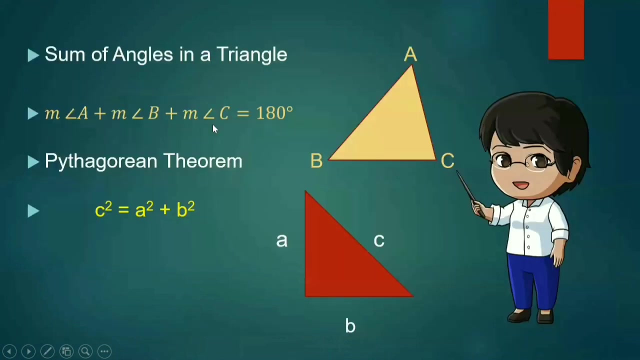 The volume of a cylinder is equal to r squared H, the volume of a cone is one-third pi? r squared H, or one-third of the volume of a cylinder with the same height and radius. and the volume of the sphere is equal to four-thirds pi? r cubed the sum of the angles in a. 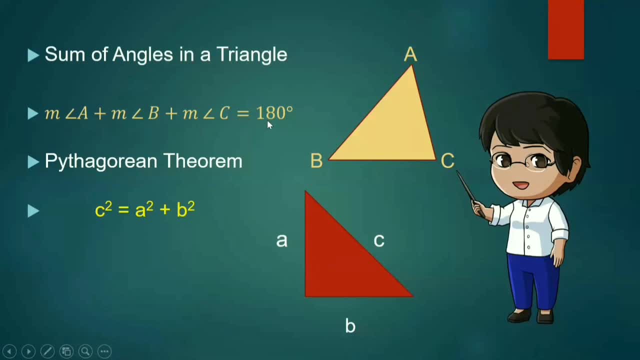 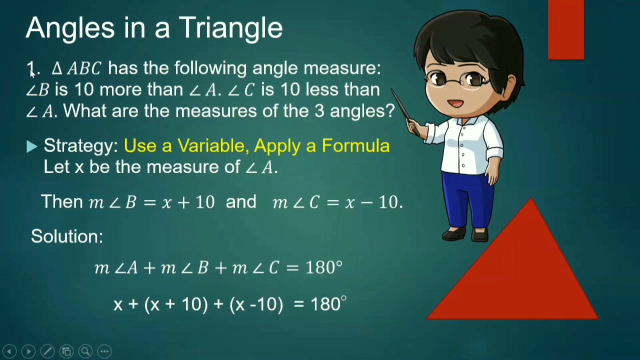 triangle is equal to 180 degrees and the Pythagorean theorem, c squared is equal to a squared plus b squared, where c is equal to the hypotenuse and a and b are the legs of a right triangle. let's have some examples. number one: triangle. 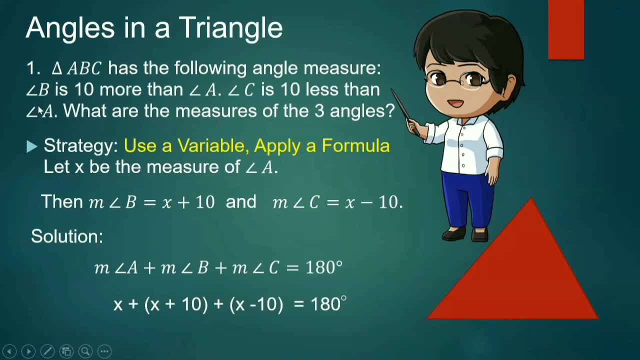 ABC has the form of a triangle and a triangle has the form of a triangle and the following angle measure: angle B is 10 more than angle a and angle C is 10 less than angle a. what are the measures of the three angles? strategy: use a. 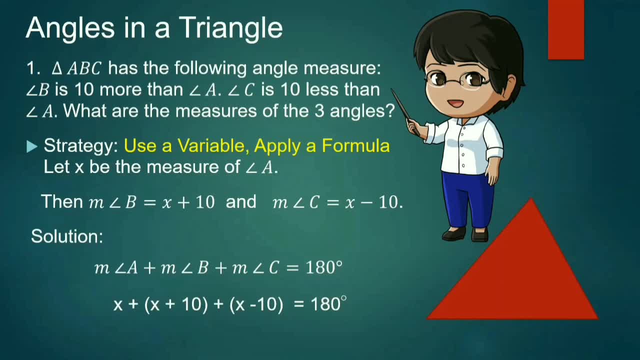 variable and apply a formula. so let X be the measure of angle a, then the measure of angle B is equal to X plus 10 and the measure of angle C is equal to X minus 10. so adding the three angles we have X plus X plus 10. plus X minus 10 is 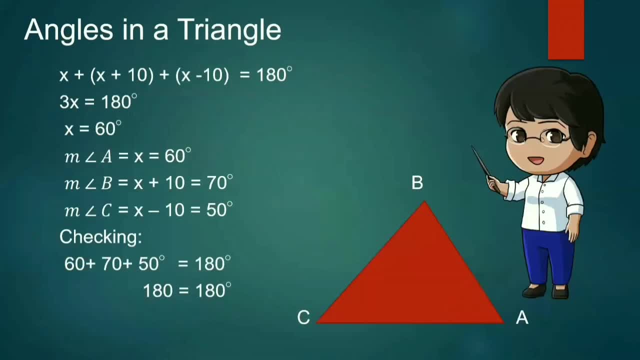 equal to 180 degrees. so we add this 3 and we have 3. X is equal to 180 degrees. dividing both sides of the equation by 3, we have X is equal to 60 degrees. therefore, the measure of angle a is equal to 60 degrees. the measure of angle B is equal. 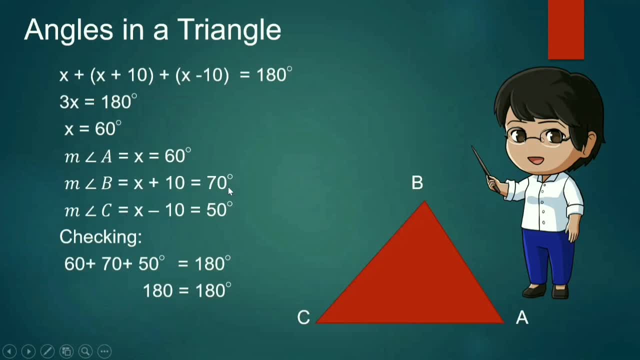 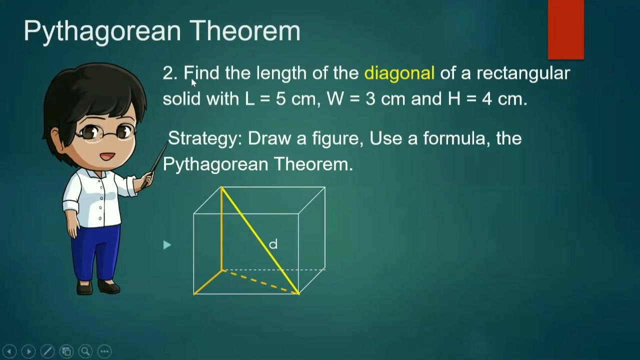 to 60 plus 10 or 70 degrees and the measure of angle C is 60 minus 10 or 50 degrees. checking getting the sum of the three angles, we have 180 degrees. problem number 2: find the length of the diagonal of a rectangular solid with length is equal. 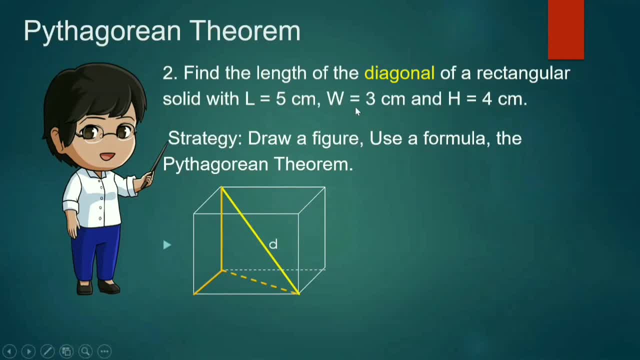 to 5 centimeters, width is equal to 3 centimeters and height is equal to 4 centimeters. so the strategy is to draw a figure, use a formula, and the formula that we will use here is Pythagorean Theorem. if you look at the figure, 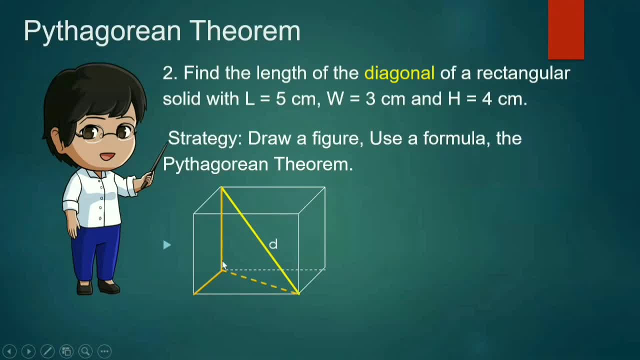 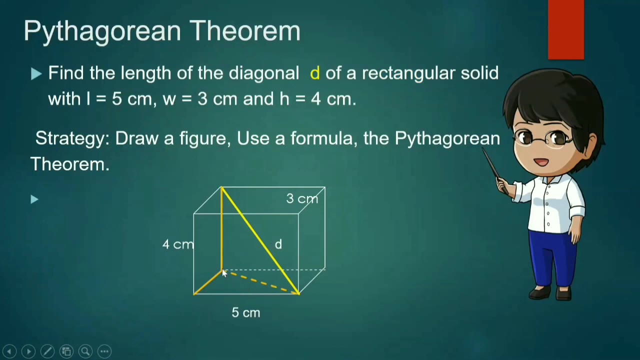 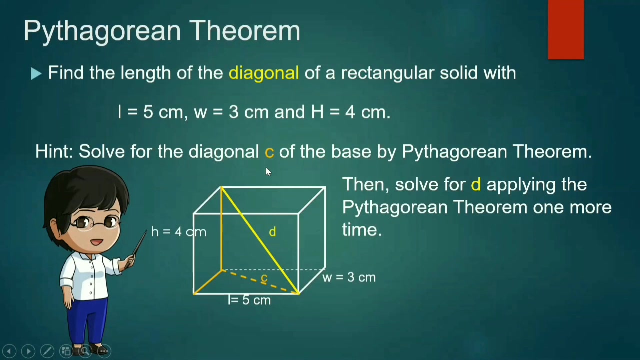 Here we have a right triangle here at the bottom and another right triangle here which is standing. so we will solve for D, but we have to look for the value here of this hypotenuse which we will call C, so solving for the diagonal C of the base by Pythagorean theorem. and then we also 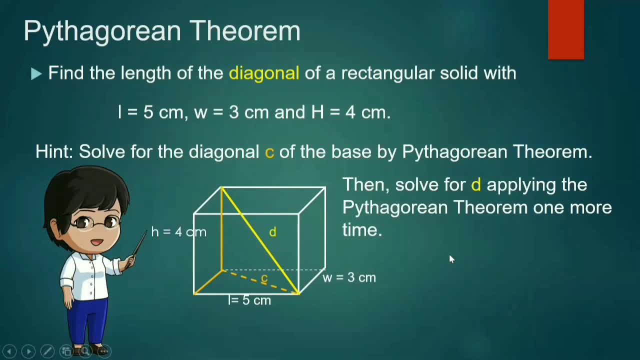 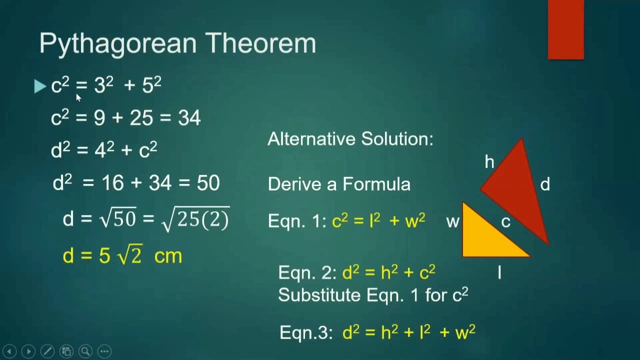 solve for the diagonal D one more time using the Pythagorean theorem. solving for C, we have: C squared is equal to 3 squared plus 5 squared. so C squared is equal to 9 plus 25 squared is equal to 34. then, solving for d squared, we have: d squared is equal to 4 squared plus c squared. 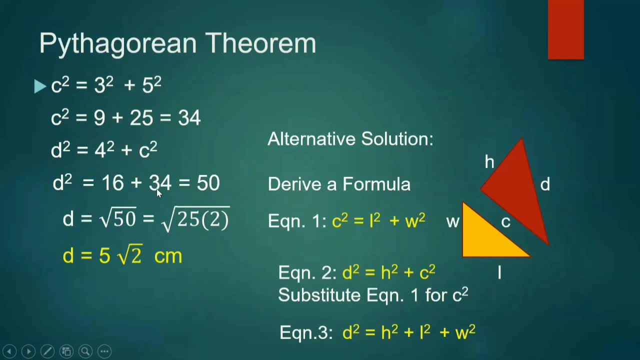 and d squared is equal to 16 plus 34 is equal to 50.. the square root of 50 is equal to 5 square root of 2 centimeters. and we have an alternative solution. we can derive a formula so that we will have one formula for the whole problem. so equation one is for the formula for c. c squared is equal to. 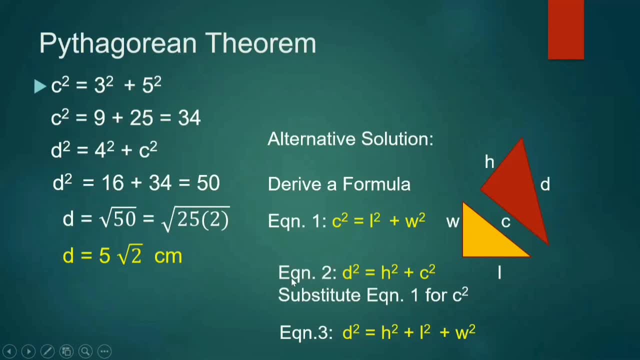 l squared plus w squared. and then equation two is the formula for d: d squared is equal to h squared plus c squared. then substitute equation one for c in equation two and we get equation three, which is: d squared is equal to h squared plus l squared plus w squared. 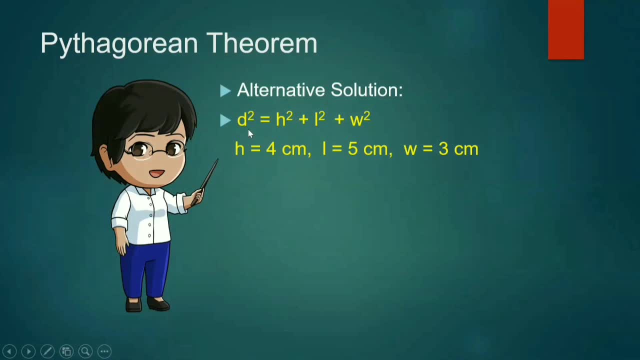 the alternative solution is: d squared is equal to h squared plus l squared plus w. with the given values we have d squared is equal to 50, and then d is equal to square root of 50, or d is equal to 5 square root of 2 centimeters. 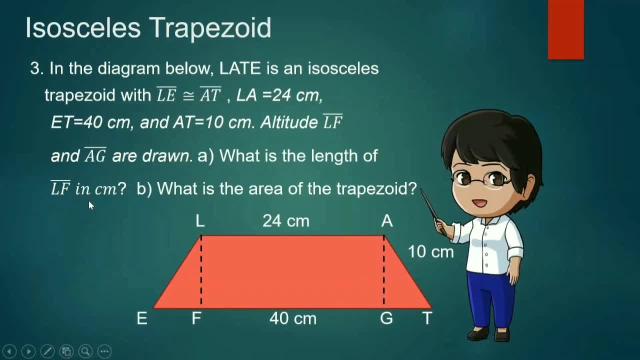 problem number three: in the diagram below, lat is an isosceles trapezoid with le congruent to 80, and la is equal to 24 centimeters, the first base- and et, the second base, is equal to 40 centimeters. so, uh, the altitude, lf and ag are drawn, so we have 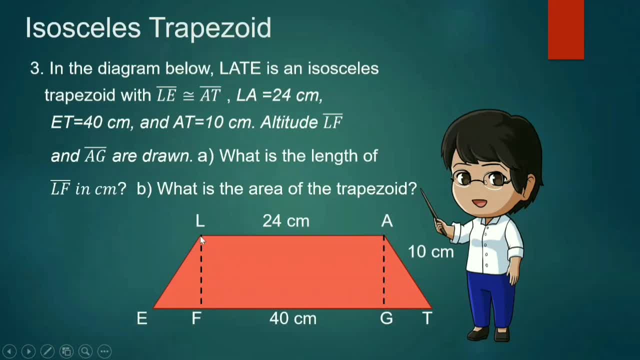 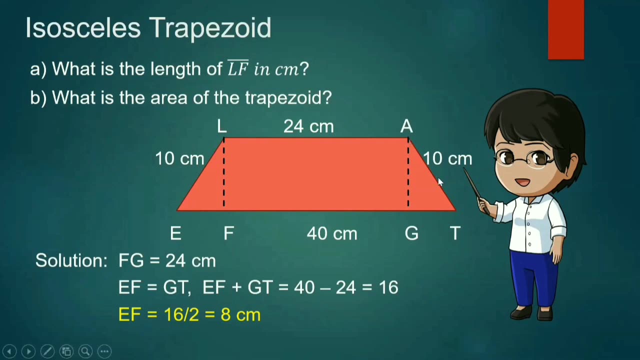 lf and ag, what is the length of lf in centimeters and what is the area of the trapezoid? so, since the trapezoid is an isosceles trapezoid, we have 80 is equal to le or le is equal to 10 centimeters. and then, since we have 24 here, la is 24 and la is parallel to. 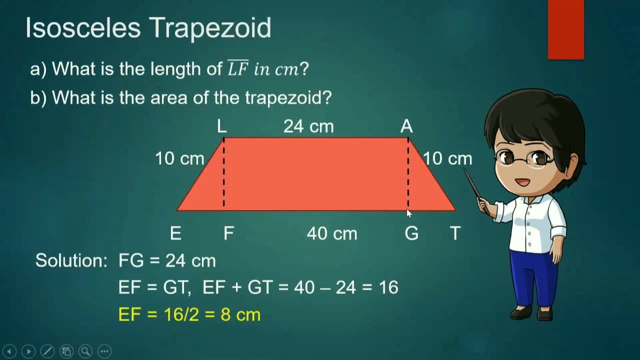 fg. so fg here is also 24, leaving this line segments ef and line segment gt as the difference between 40 and 24. so we get the values of ef and gt, since they are also equal. we have: ef plus gt is equal to 40 minus 24 is equal to 16.. and then 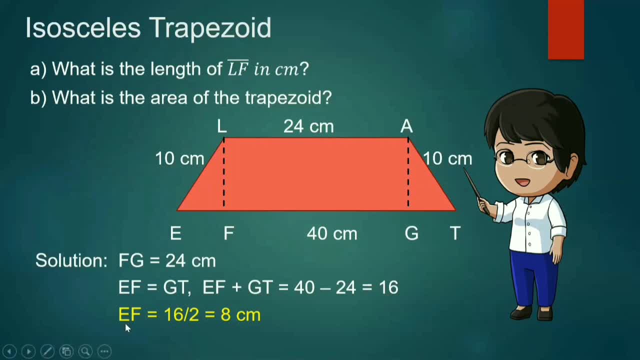 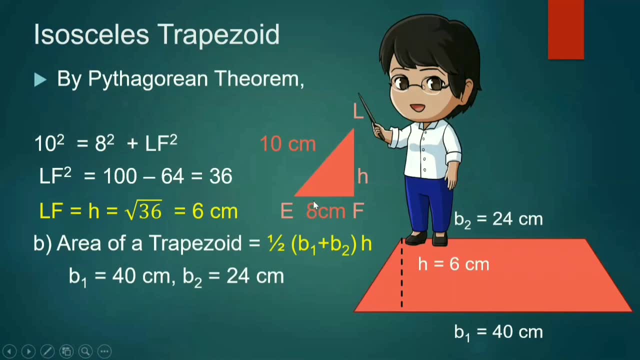 dividing 16 by 2, we get the length of ef, which is 8 centimeters. then we will just simplify the figure by getting the triangle and from this part. so we have eight centimeters and then 10 centimeters for our hypotenuse. so we will solve for. 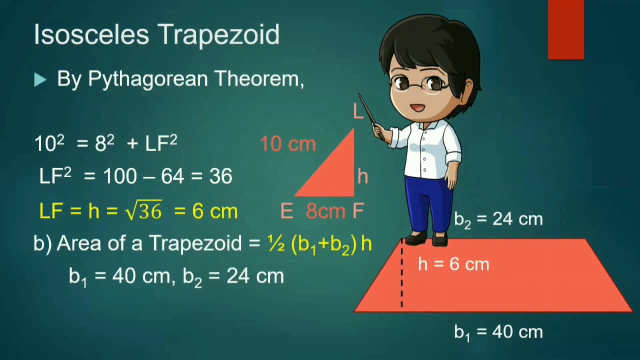 lf and using the pythagorean theorem we have: lf is lf. squared is equal to 100 minus 64 is equal to 36. so l? f is equal to square root of 36 or six centimeters and the area of the trapezoid is equal to one half of the base one plus base two. 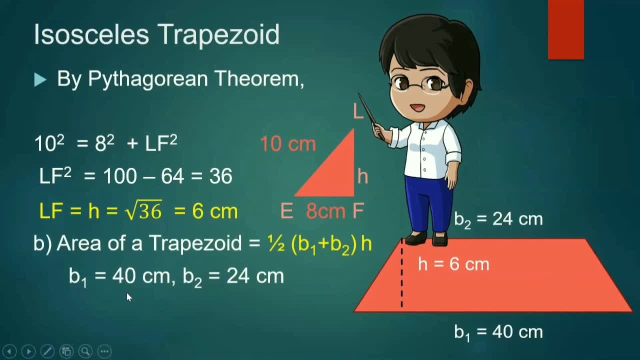 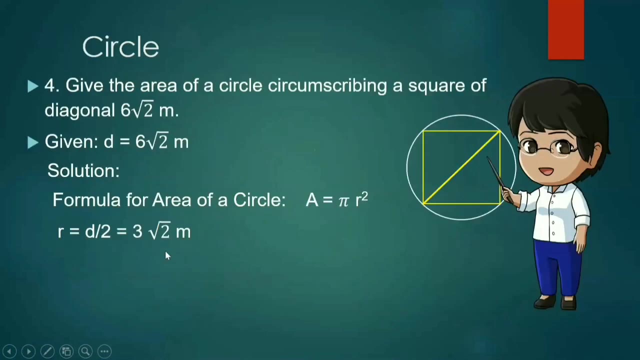 times the height, since base one is equal to 40, base 2 is equal to 24, then 1 half of 40 plus four times the height, six is equal to 196 centimeters. problem number four: give the area of a circle circumscribing square of diagonal six square root of two. 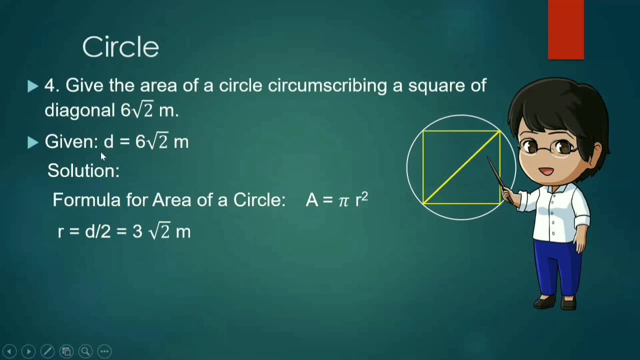 meters. so we have a given diagonal, six square root of two meters, and we know that half of the diagonal is equal to the radius. so here is the solution: the formula for the area of the circle is equal to PI R squared, and our radius is three squared of two meters. so the area of the circle circumscribing the square 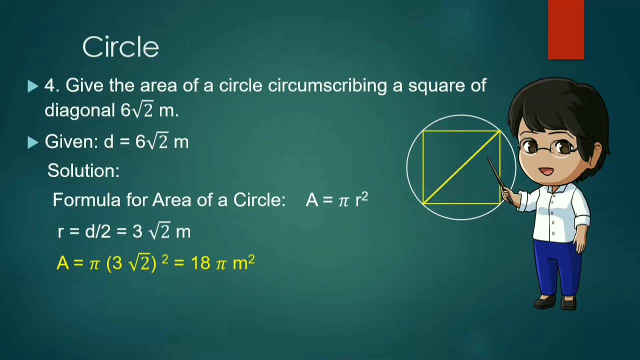 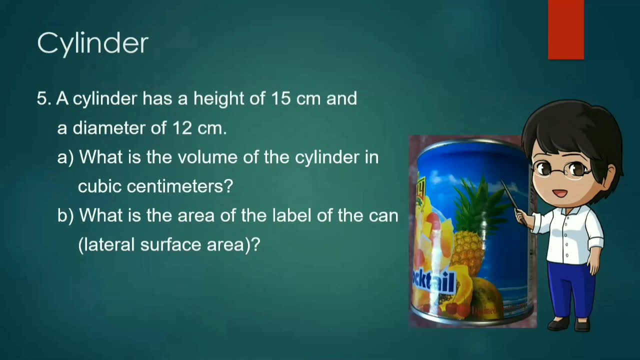 is equal to PI squared square root of two times three squared, or 80 in PI meter squared. problem number five: a cylinder has a height of 15 centimeters and a diameter of 12 centimeters. what is the volume of the cylinder in cubic centimeters and what is the area of the label of the can or? 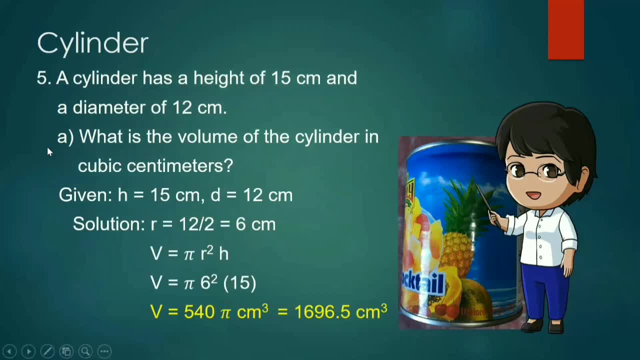 the lateral surface area. so first we find the volume of the cylinder in cubic centimeters. we have the height given. height is 15 centimeters and the diameter is 12 centimeters. so we will divide this by 2 and we have a radius of 6 centimeters. so the formula for 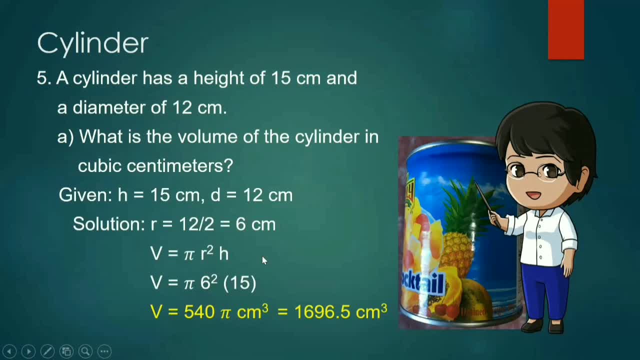 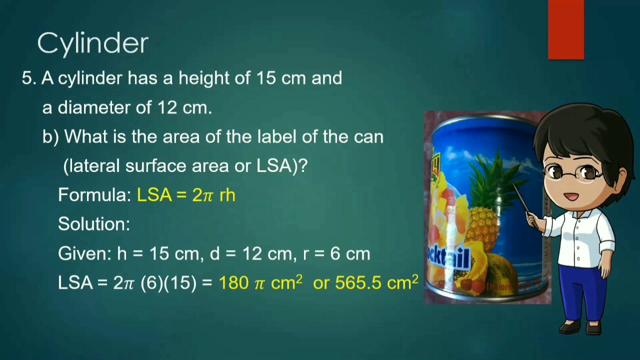 volume is pi r squared times h and we get the volume is 540 pi centimeters cubed, or 1696.5 centimeter cube. then for letter b, what is the area of the label of the can, or the lateral surface area? the formula is 2 pi r times h, or the circumference of the circle times the height of the can. 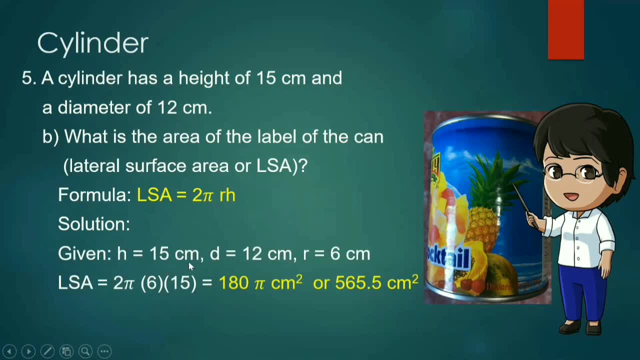 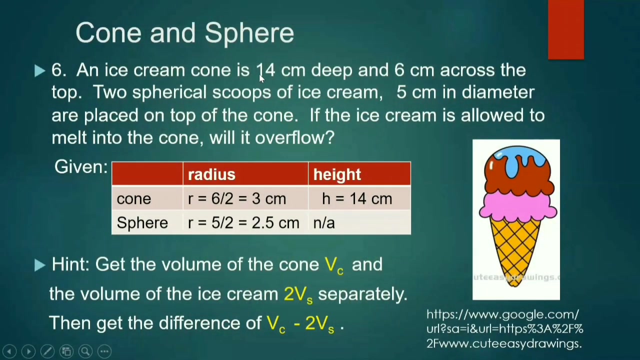 so, given h is equal to 15 centimeters and r is equal to 6 centimeters, the lateral surface area is equal to 180 pi or 565.5 centimeters squared. problem number six: an ice cream cone is 14 centimeters deep and six centimeters across. 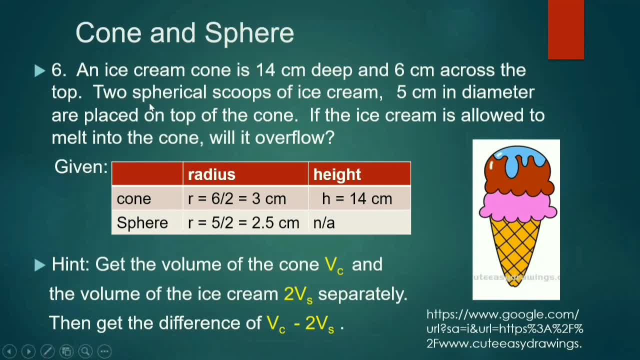 the top, two spherical scoops of ice cream five centimeters in diameter are placed on top of the cone. if the ice cream is allowed to melt into the cone, will it overflow. so the given is the diameter of the ice cream cone. so we get the radius from there. we divide the ridge, the diameter.